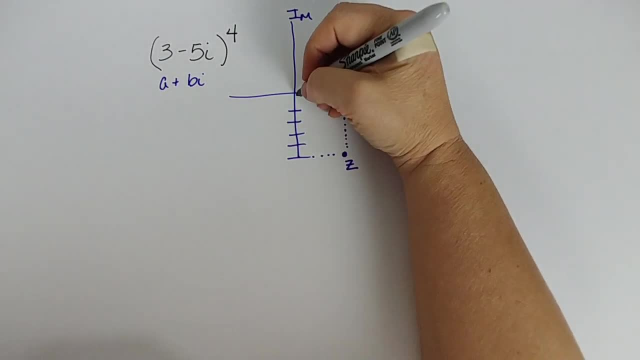 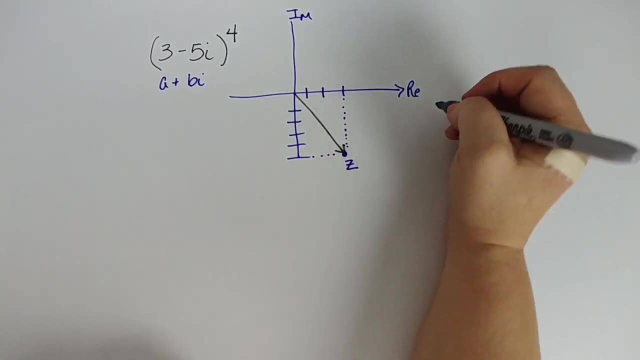 Okay, so what do we mean by that? Well, we could write this: The distance is a vector distance from the origin. Okay, so also written as magnitude of z. You notice it's in absolute value, bars, because think about this, This distance really is the absolute value of z, It's how far it is from 0.. 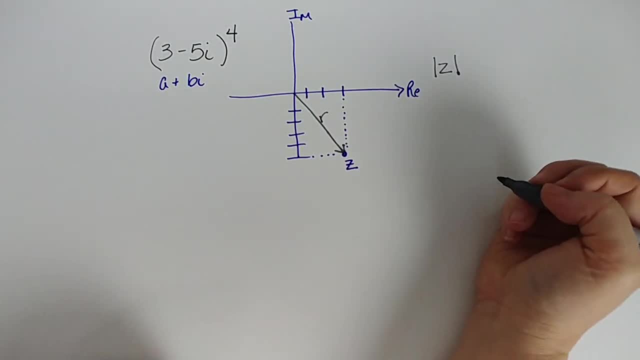 Okay, and so we call that r and it's actually also called the modulus. That's one of the worst things about math: You have five different names Sometimes for things sometimes, and the definition doesn't change. Sometimes we give it different names, But it's the. we'll call it the r value. Okay, and when you think of circular distance, 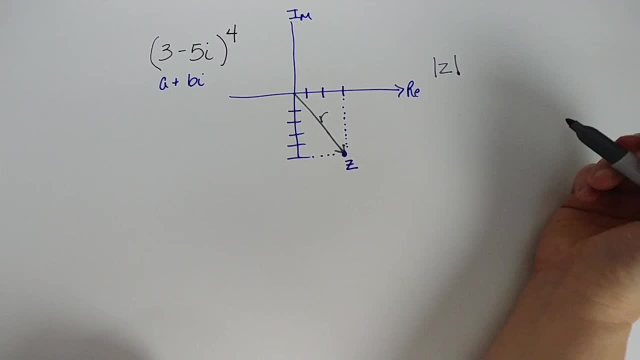 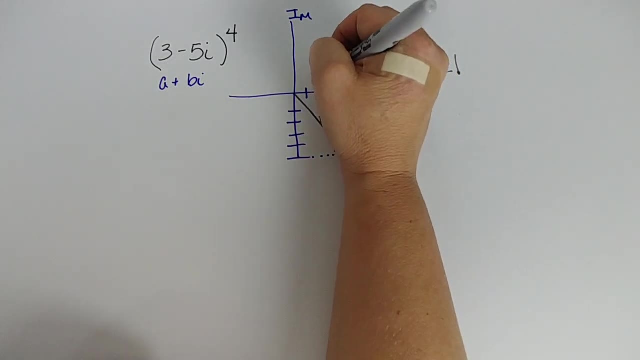 a lot of people call that radius. It'll probably happen in this video where I will call it radius. So think about this: We have this triangle right. We have a right triangle. We have a distance here a. We have a distance here b- Right triangle. if you don't see it, there's your right angle. 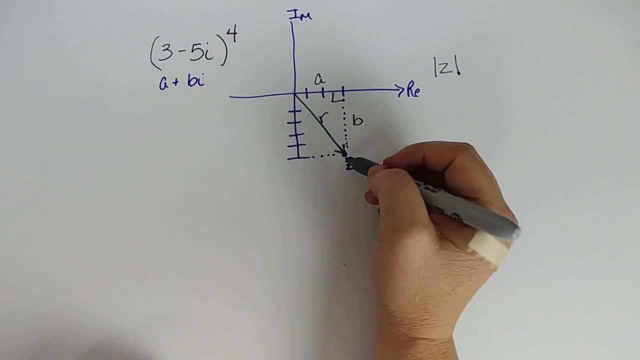 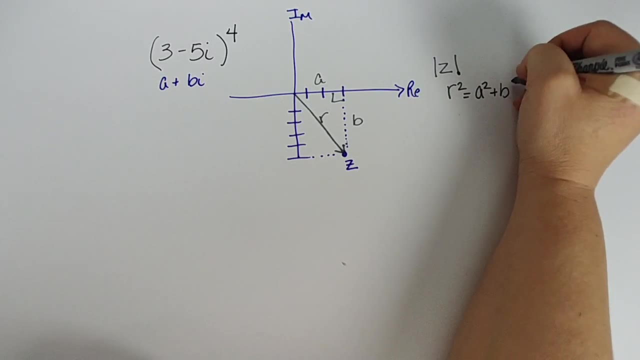 R is our hypotenuse. So I can find this distance with what I've been given, because I know that r squared is equal to a squared plus b squared right, Because I know the Pythagorean theorem since like the seventh grade. So then I know that this distance is going. 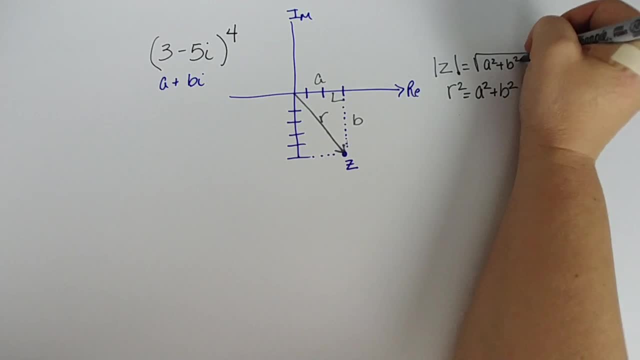 to be the square root of a squared plus b squared. Well, great, That's distance. I did mention that we need a distance and direction. So let's talk about direction. If I told you to go r distance from the origin, there's so many ways, infinitely many ways you can do that You're not going to get. 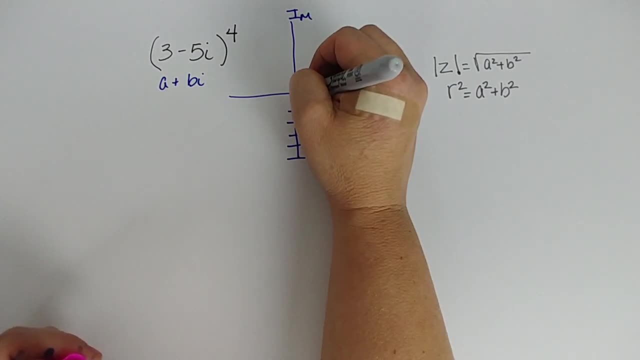 to the right point. I mean, you might guess, but I doubt it. Okay, So we need direction. theta Direction is our angle, It's the angle created by this vector here, this little distance here, and the positive x axis. Okay, So we can find that. All right, We know we have a right triangle, We know angles. 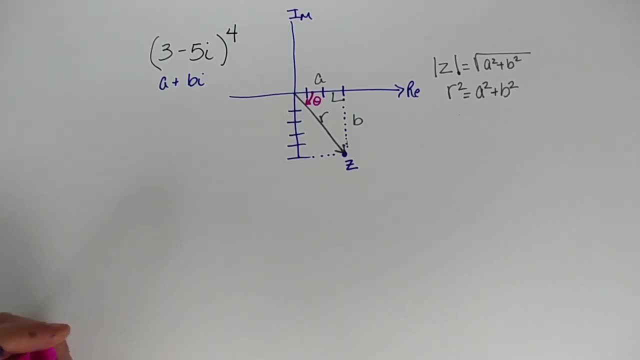 involve SOHCAHTOA, right, Sine, cosine and tangent. That's not going to go away. So let's start looking at some of our relationships. Actually, let's talk about what we're going to do, What theta is going to be All right. So if we have SOHCAHTOA- yeah, I still write it down- And we 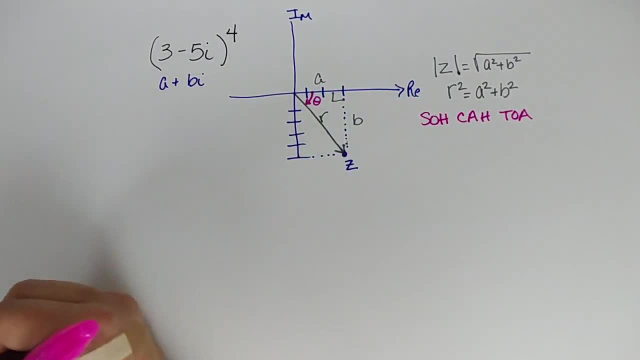 have this angle. Well, we know we have the opposite and we have the adjacent. So which one of those deals with opposite and adjacent, And that is tangent. So I know that the tangent of theta is going to be opposite, which is b over adjacent, which is a. So the tangent of my angle is b over a. 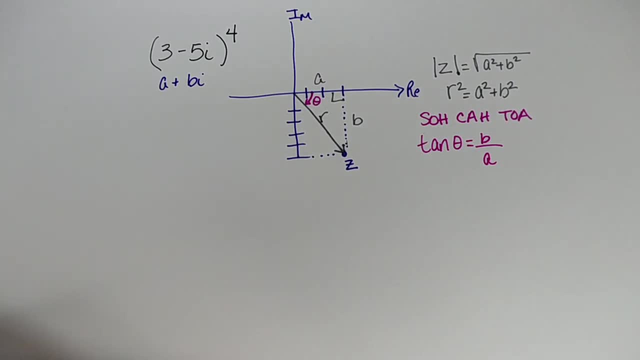 Okay, Let's take it one step further. I know that when I solve for angles, I use inverse tangent or arc tangent. So then I know that theta is going to be the. I'm going to write it as inverse or arc tangent, b over a. Okay, Great, Now we want to manipulate a and b. We want to talk about what a. 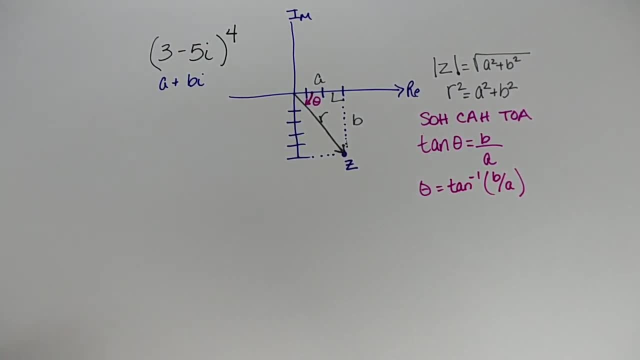 and b mean in terms of cosine, sine and tangent. All right, So let's look at this and let's get one more color. Let's have a rainbow on here, But if you look at our angle, okay, then let's do a first, because a 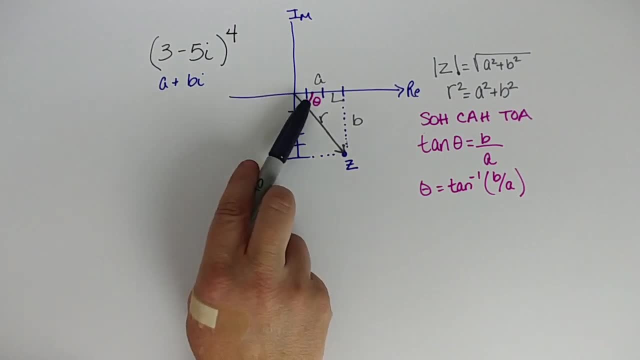 comes first here in our a plus b i form: Okay. So let's look at a. Okay, A is adjacent, And I know cosine, right, Cosine is adjacent over hypotenuse. So then I know that the cosine of a, nope. 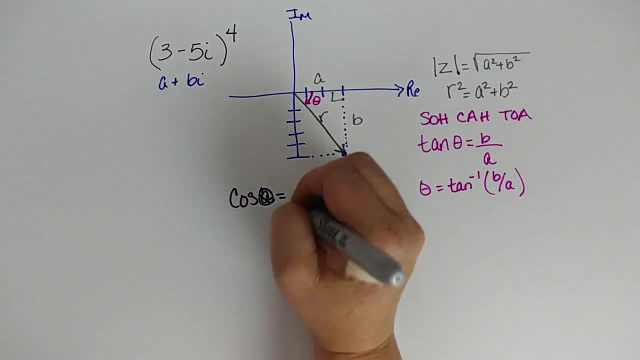 cosine of theta. that didn't look right. Cosine of theta is a over r. Got a little ahead of myself, Okay, So the cosine of theta equals a over r, which, if I remember, I only care about a, I want to solve for a. So I'm going to multiply both sides by r And that gives me what. 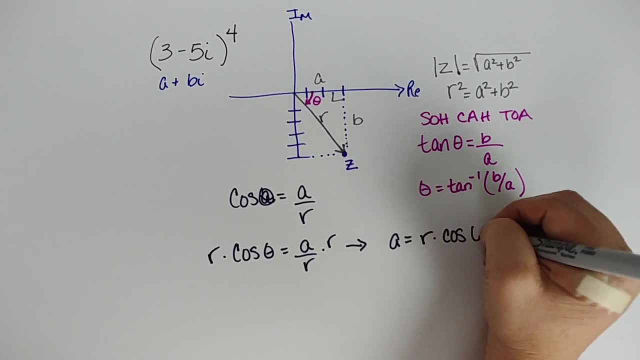 a equals r times the cosine of theta. And you're probably thinking I bet you can do the same thing for sine. And you can, as long as you don't mess up and say the sine of a or the sine of b. Okay, 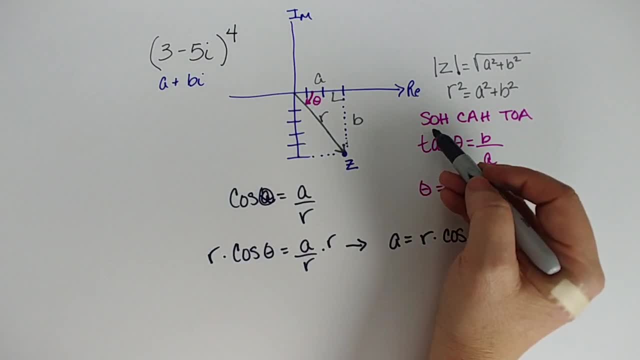 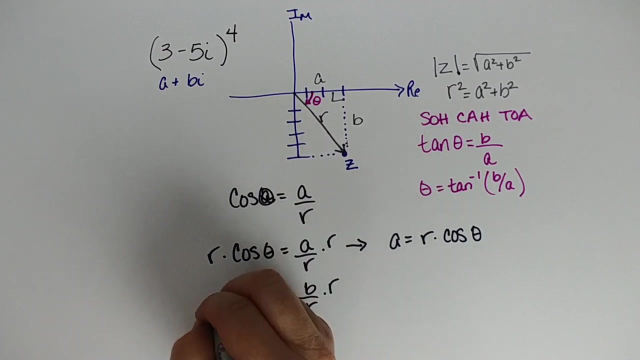 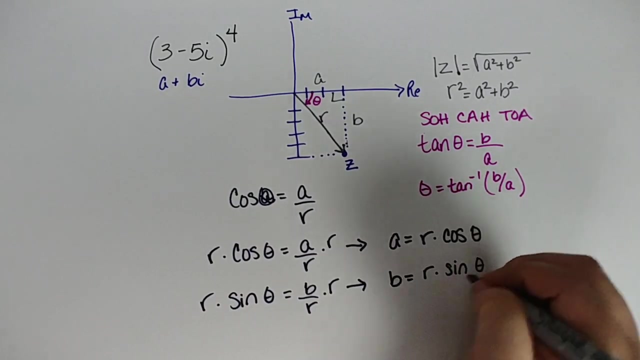 b is my opposite over hypotenuse, I know so is opposite over hypotenuse, right? So I know that the sine of theta is going to be equal to opposite b over r. Yes, I'm going to multiply both sides by r And I'm going to say that b equals r times the sine of theta. Great, Now I can put this all. 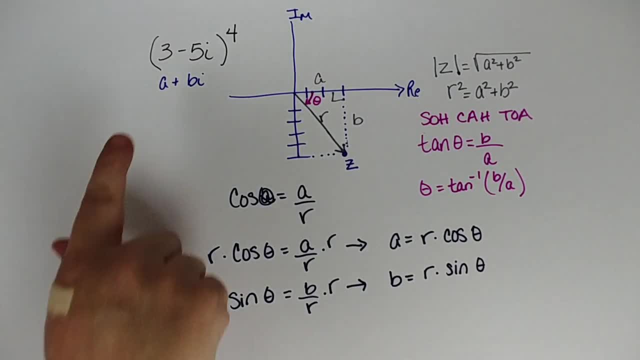 together. I have to do some calculating still, But I really can't. So I'm going to take my a plus b i form here, And I'm going to get rid of a And I'm going to get rid of b, Because in polar form we don't have a and b. So what's my a? 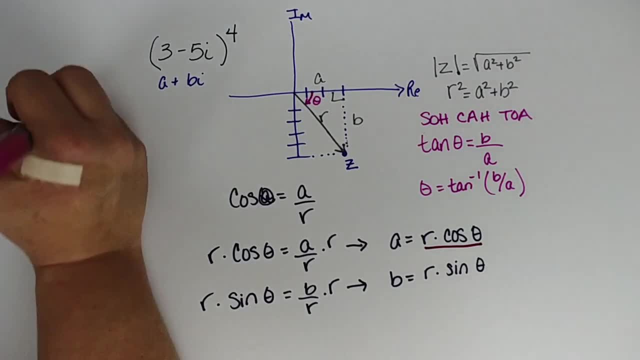 r times cosine theta. So I'm going to write that r times cosine theta plus instead of b. what's b? r times sine of theta? Remember, this is our imaginary part, So we get the. i Don't lose that. 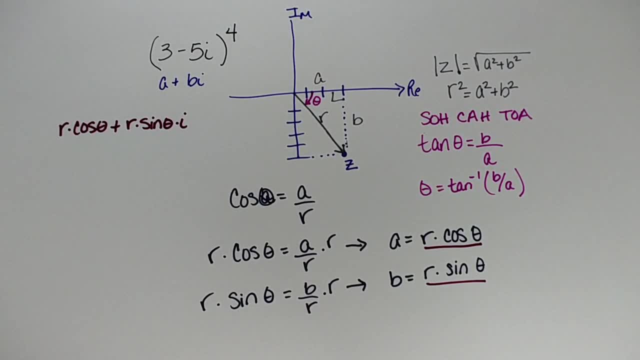 All right, And you know, you've been in math how many years. You know we're not going to let you leave it like this. We're going to factor out the r, which gives us r times, cosine, theta plus, bring out the i. 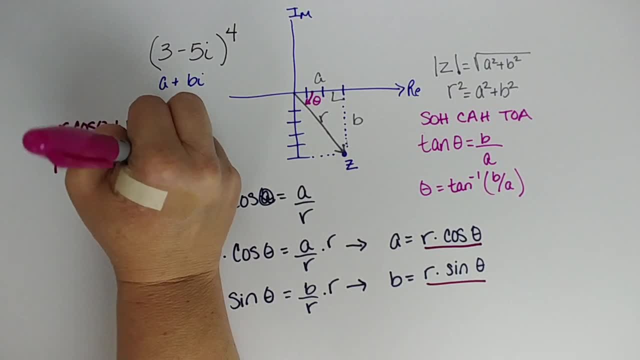 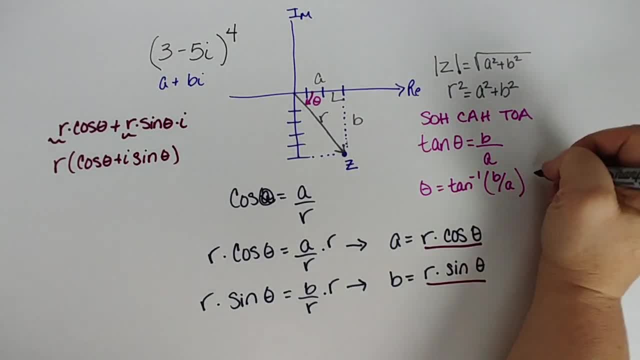 Let's actually put some numbers into that, Let's get some values, All right. So that means that this is the inverse tangent of negative five over three, Right, Okay, We're going to put that into a calculator, because I don't know what that is And you know, these numbers aren't very nice. A. 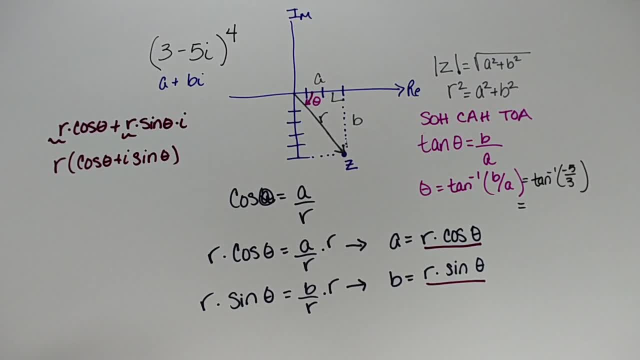 lot of times you see these complex numbers and they're written with rad three over two or one half, or rad three is your a and your b value And those are really nice radian numbers. This is not Okay. Three and negative five are not nice radian numbers. 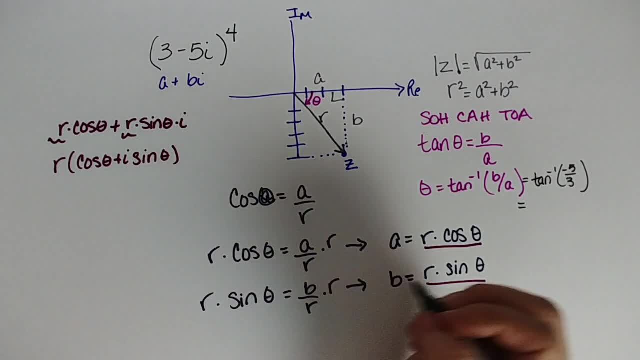 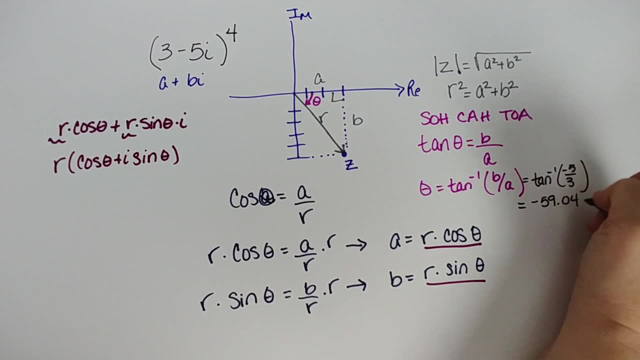 So I'm going to do this in degrees, Okay, So be sure you know what mode your calculator is in, And you get negative 59.038.. So we'll say zero four. We're going to go to the hundredth place. 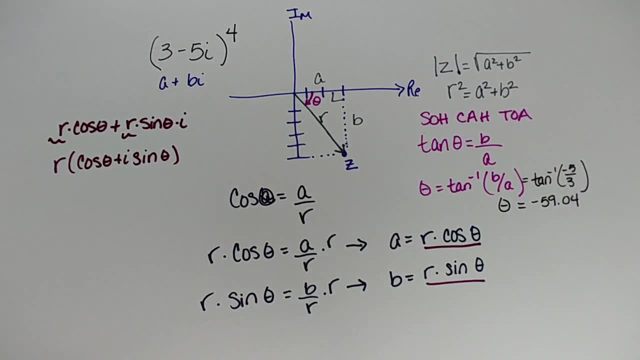 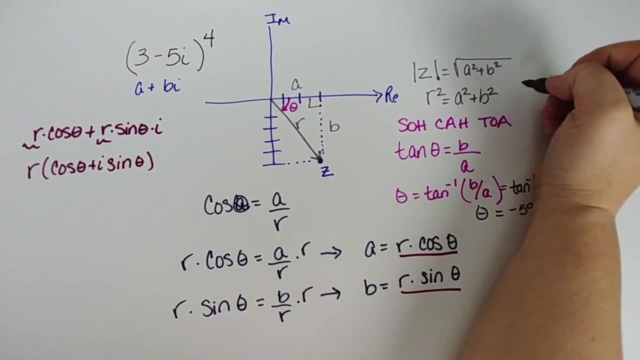 So that is what my theta is. Okay, Now I need to solve for my r value, Okay. Well, I told you way up here that r. can you see that? Okay, So it was the square root of a squared plus b squared. 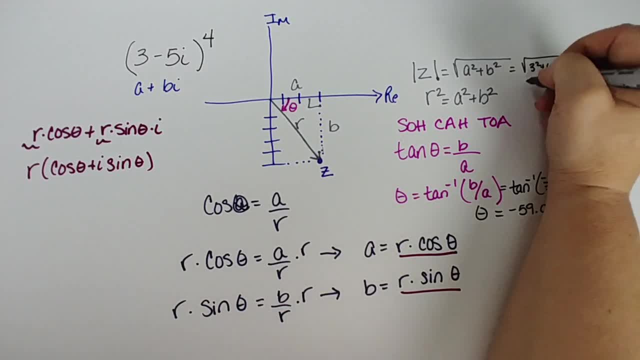 So three squared plus negative five squared, So that's going to be nine plus 25.. So rad 34 is our r value. Okay, All right, So now we kind of have everything we need. We can plug this all in, All right So. 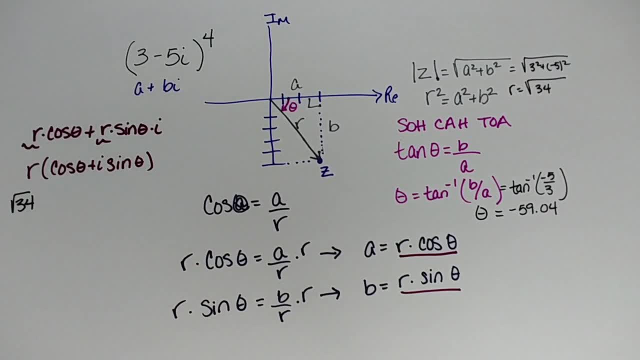 r right here, squared of 34, cosine of theta, Okay, So cosine of negative 59.04.. Plus i times the sine of that same angle. And what did this problem want us to do from the get-go? It wanted us to take this whole thing. 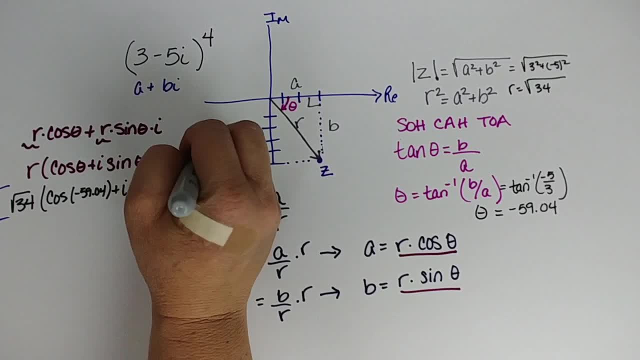 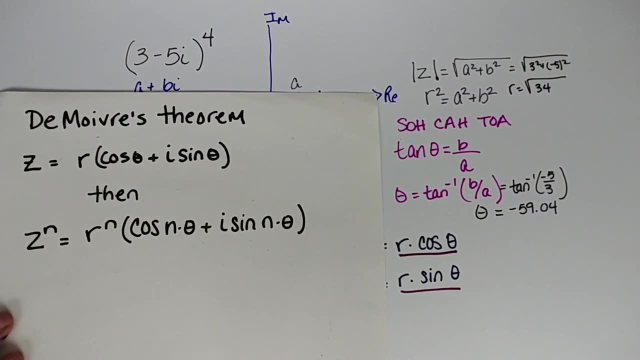 and raise it to the fourth power. All right, So now, lo and behold, we can use that theorem that we were asked to use in the very beginning. We can simply raise our magnitude to that power and multiply both angles by that same number. Okay, So this is getting better. 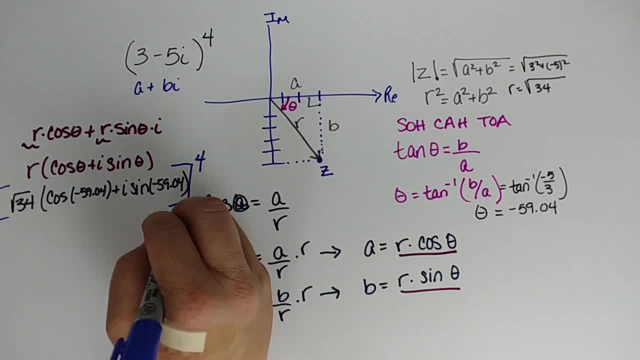 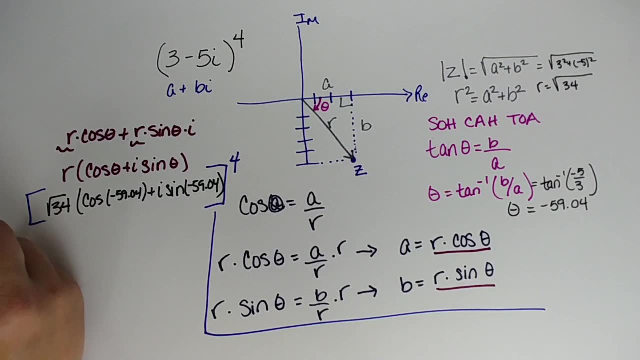 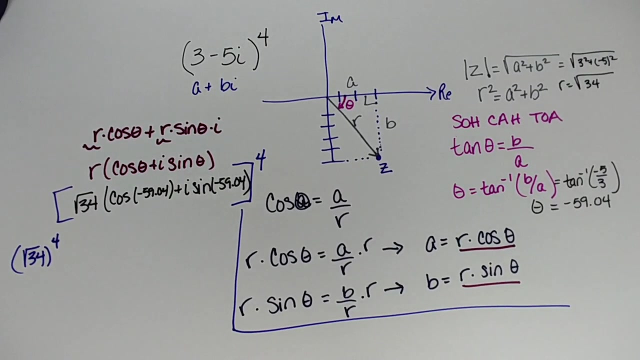 So we are going to have- let's kind of coordinate my work off and maybe move this over a little bit. Okay, So we're going to have rad 34 raised to the fourth power And we're going to move it a little more because you still can't see it, And then we are going to 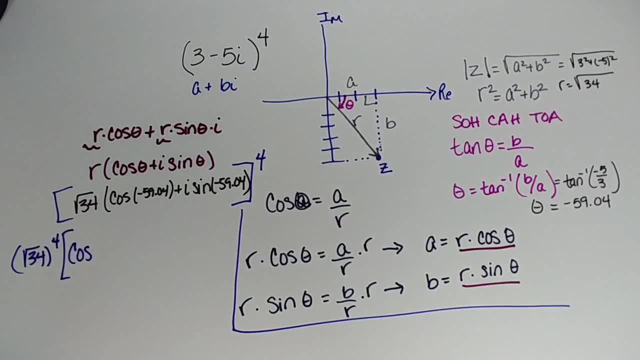 have times. I'm going to use my brackets here, cosine, What do we have? So remember I have n is 4.. So 4 times negative 59.04.. Okay, and we're going to do the same thing to our sine value. 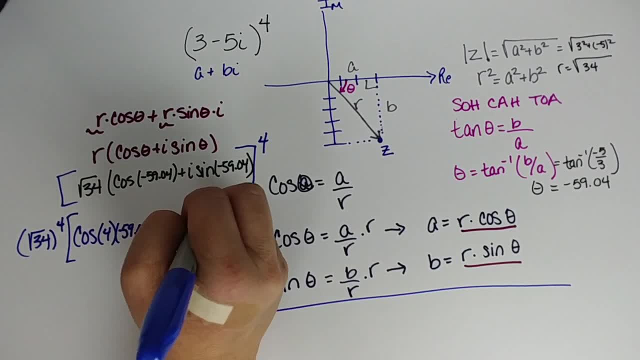 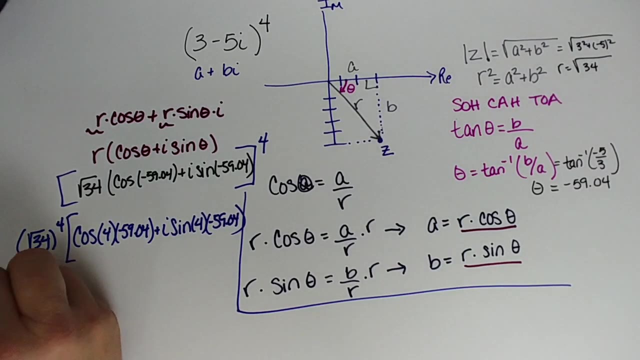 So plus i times the sine of 4 times negative 59.04.. All right, great, We're getting a little smushed here, but the calculator is going to help everything be better now. So rad 34 raised to the fourth power, when you punch it in you get 1156,. okay, times the cosine. 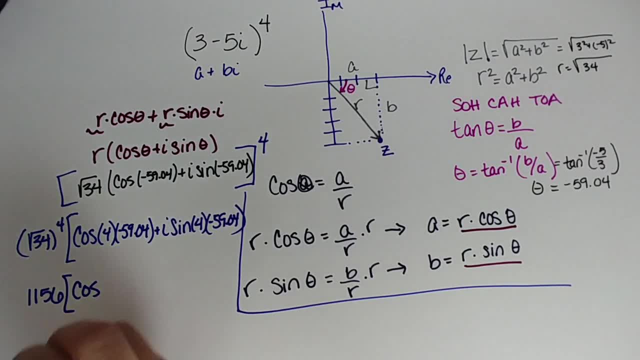 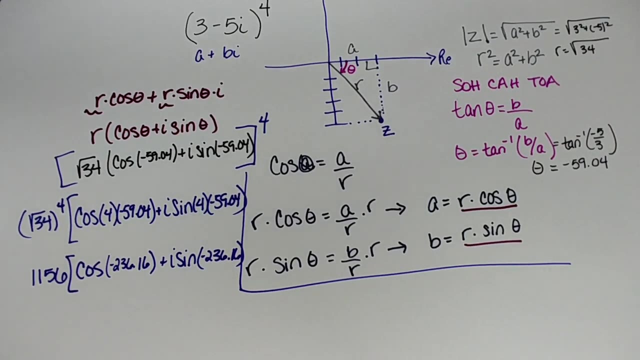 We're going to have a negative right. Negative 59.04 times 4 is going to give us negative 236.16, plus i sine of the same dang thing, negative 236.16,. okay, Well, all right. it said rectangular form, right. 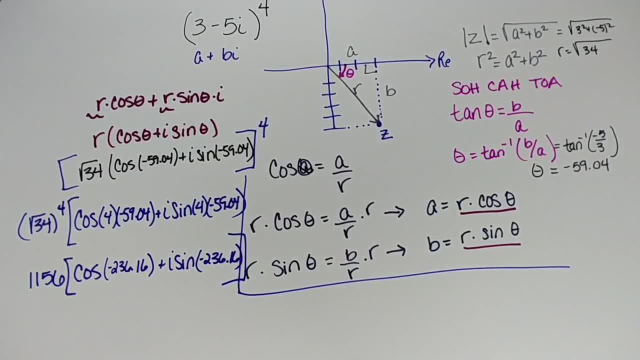 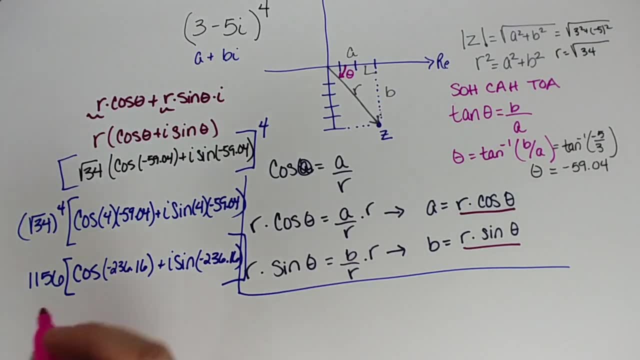 This is now polar form, albeit it's ugly. So when you want to get from here back to rectangular, all you have to do is evaluate your cosines and sines. This is actually the easy part. So you're going to evaluate the cosine at negative 236.